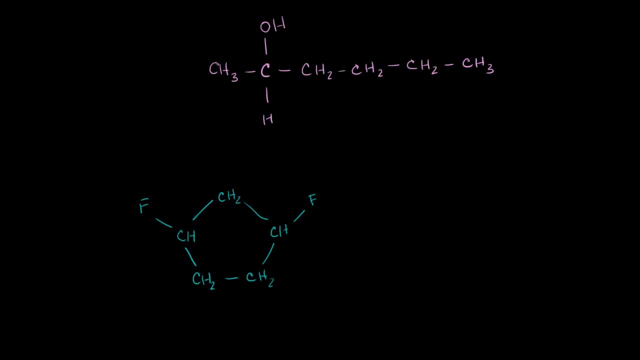 Let's do a few more examples of seeing if either an atom or an entire molecule is chiral. So here I have a molecule. Let's see if we can identify any chiral centers or any chiral atoms or asymmetric carbons. All words for the same thing, although I guess you could. 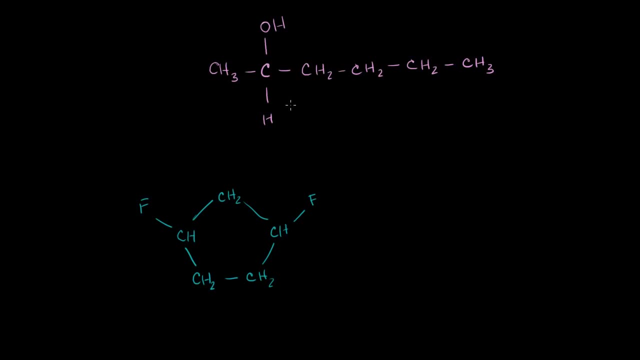 have chiral centers that aren't necessarily carbon, But it tends to be carbon most of the time, especially in an organic chemistry class. So if we look here, the one that kind of jumps out, this carbon right here is bonded to three hydrogens and another. 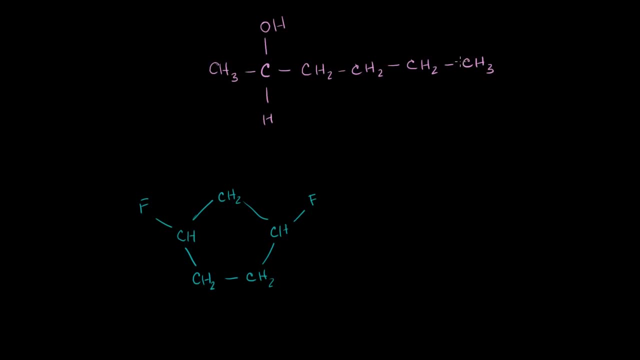 carbon, so this is obviously not going to be a chiral center. it's bonded to three of the same group. These three guys are all bonded to two hydrogens each. so they're all bonded to two of the same group. so they 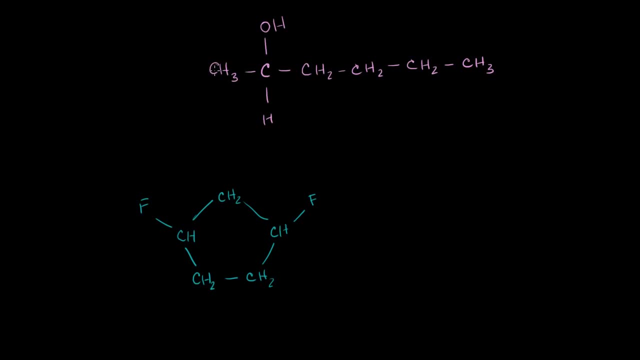 can't be chiral centers. This carbon right here is bonded to three hydrogens- Once again, three of the same group, not going to be a chiral center. This one looks interesting. Looks like it could be a good candidate for a chiral center. 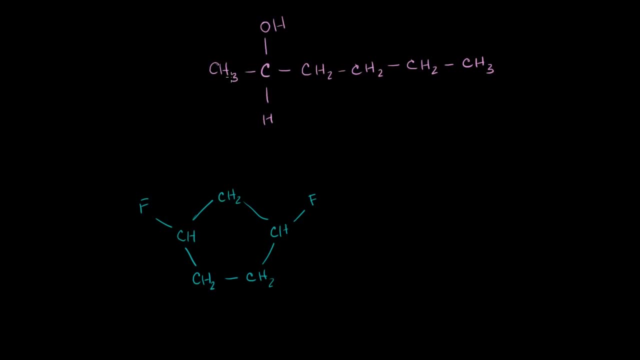 or a chiral carbon or an asymmetric carbon. Over here on the left it's bonded to a methyl group. so this is a methyl group, And here on the right it's bonded to a butyl group. Over here it's bonded to an OH, and then over here it's 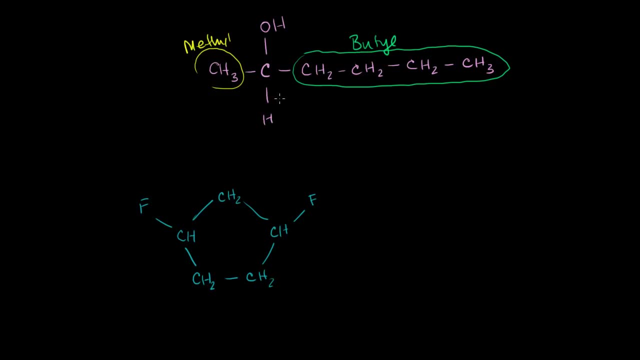 bonded to an H, So this is definitely a chiral carbon. We could put a little asterisk here. That's how they are. They often denote that this is a chiral carbon. And if this doesn't make sense to you, because you might say: 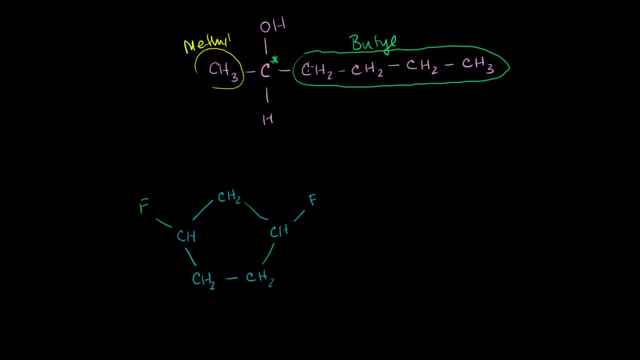 hey, Sal, look, this carbon is bonded to two other carbons. Isn't that the same thing? But the point here is that we're not looking at what atoms it's directly bonded to, We're looking at the groups that it's bonded to. 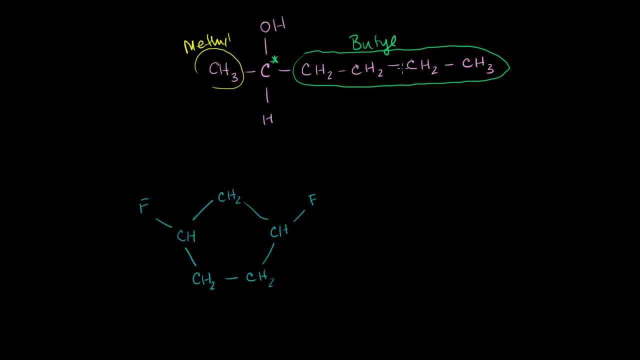 In this case, this hydrogen is a group and an atom Over here it's an entire group. It's an entire butyl group. We have four carbons here. We only have one over here. Another way to think about it, we could have drawn this: 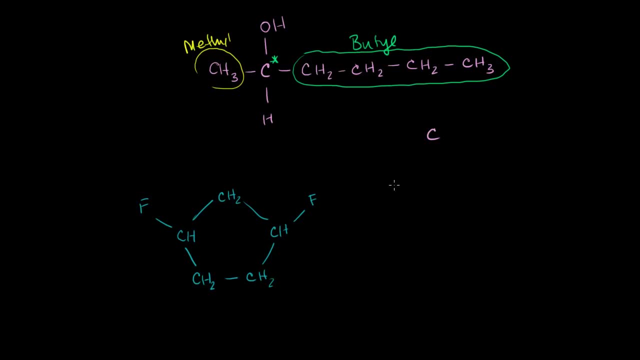 molecule Like this. We could have had a carbon in the center and maybe this methyl group is popping out like this. So maybe this methyl group is popping out like this: You have your CH3, and then you would have this hydrogen coming out, maybe in the plane. 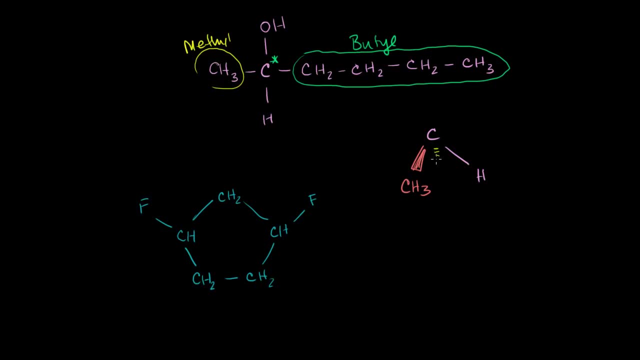 And then behind it you would have the butyl group, So kind of the back leg of the tripod you'd have a butyl. And what is that? That's C4H9,. right, That's 6 plus C4H9.. 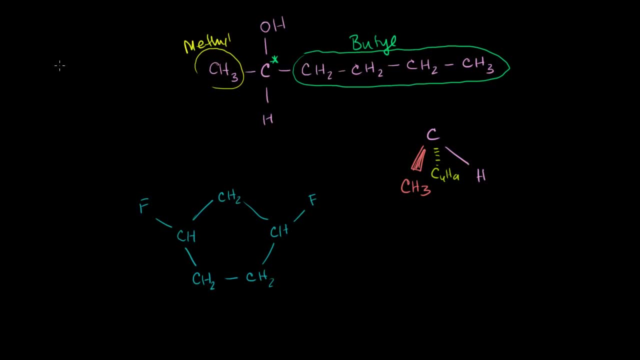 So it's C4H9. in the back And then above it you have your OH, Above it, in a different color, you have your OH, And when you look at it like this, it looks just like the other chiral carbons that we had identified in. 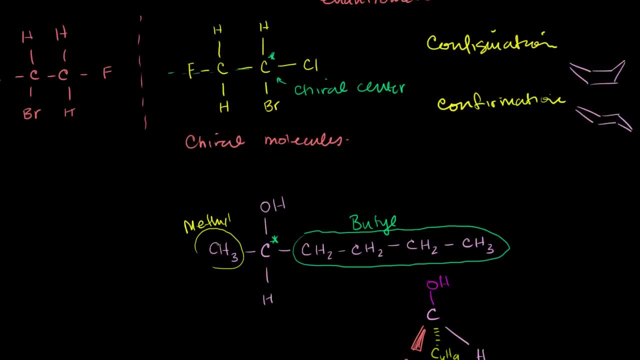 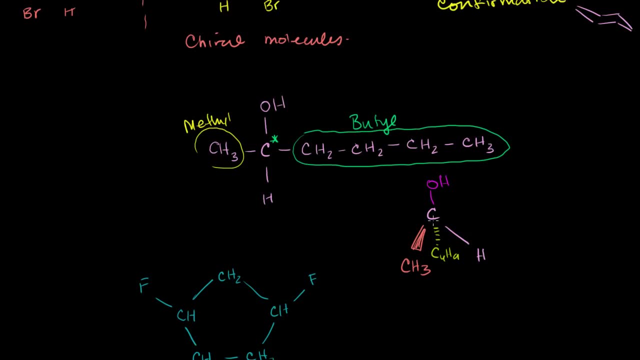 actually the last video. It looks very similar to something like this, And when you take its mirror image, this and this is the same molecule- here I kind of made it a little bit more three-dimensional, but if you take the mirror image of either one, you're going to. 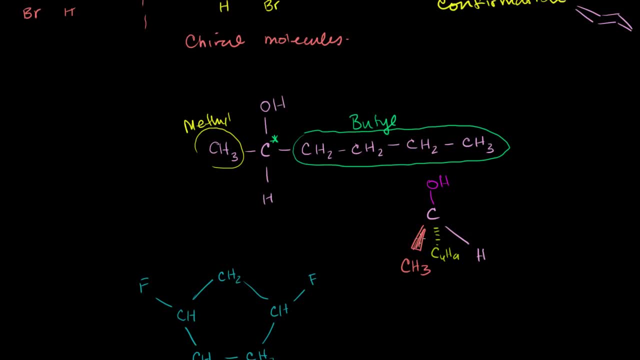 find that, no matter how you try to rotate it or shift it, you won't be able to superimpose it on its mirror image, for the same reasons as the other ones, And I challenge you to, if you can. So this is a chiral carbon. 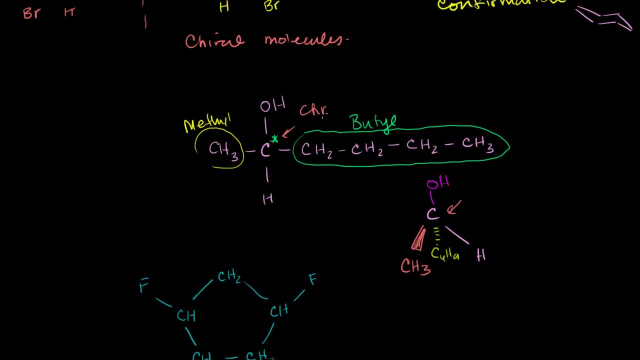 This is a chiral center, we could say, Or we could even call it an asymmetric carbon. It could be considered a stereocenter or a stereogenic center. All of those are valid things to call this carbon right there, and this is also a chiral molecule. 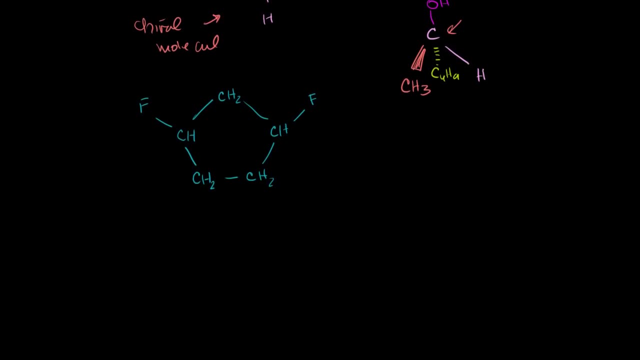 Now let's look at this blue example right here And, just as if we wanted to name it, just so we get a little bit of review, we could start at this: fluorine right there: One, two, Three, Four, Five. 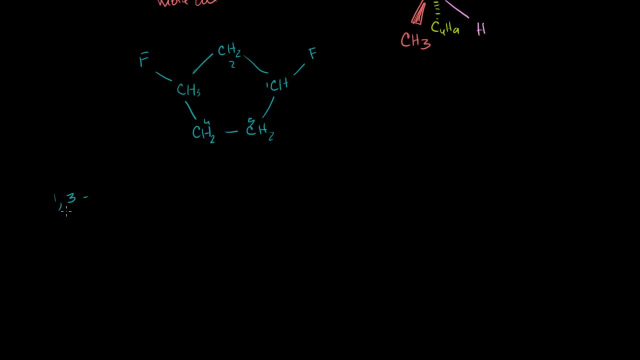 This is what This is: 1,3-difluorocyclopendane. so that was a nice review of naming, But let's think about whether we have any chiral centers here and whether the molecule as a whole is chiral. 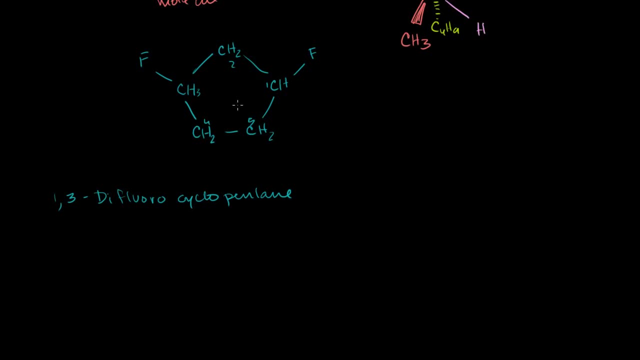 So the immediate ones that we can kind of dismiss, and actually let me get rid of this, This numbering here, just because I don't want you to think that there are somehow three hydrogens there. This is the number. that was the number: three hydrogens. 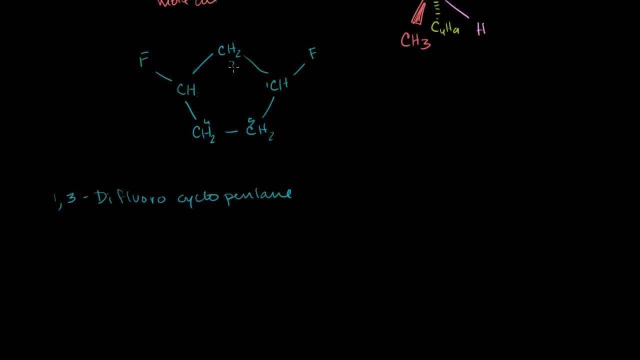 number one car- not number three carbon, number two carbon, so on and so forth. But let me get rid of them now that we've named the molecule. I don't want to confuse how many hydrogens we have at any of these points. 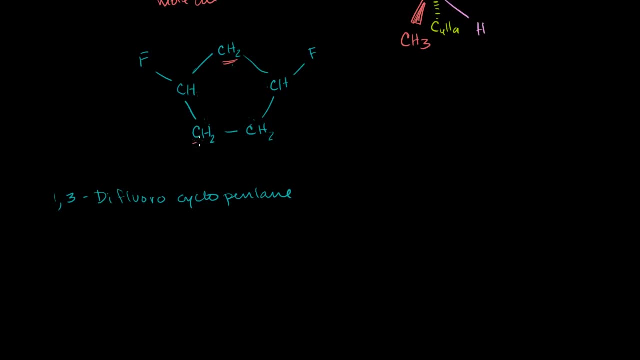 So let's look at the carbons. Well, we can immediately dismiss that carbon, that carbon and that carbon, because each of those are bonded to two hydrogens. If we wanted to break it out, they would look like this: So they're bonded to two hydrogens. 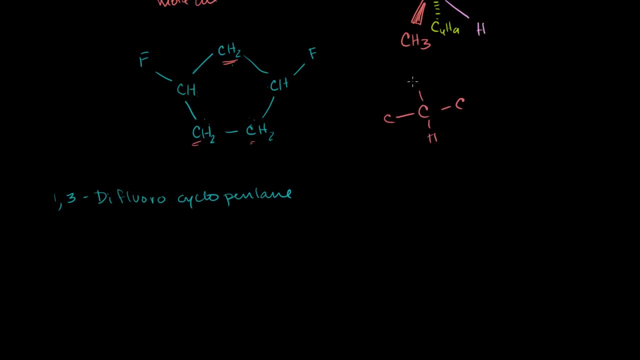 They're bonded to two hydrogens. They're bonded to two hydrogens. So they're bonded to two hydrogens. So they're bonded to carbons, carbons, and then they're bonded to hydrogens. Now, these might be different groups. 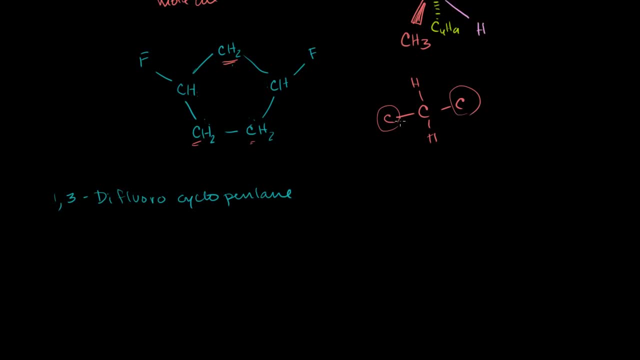 These might be different types of alkane groups that it's bonded to, So that doesn't necessarily throw it out of the running. But these two, the two hydrogens that it's bonded to, are definitely the same atom, the same group. 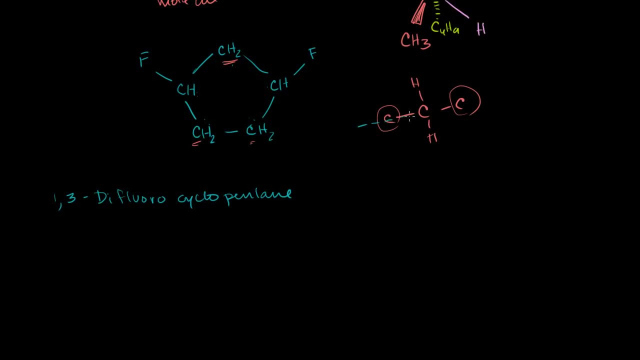 We have an axis of symmetry through that atom, So it cannot be a stereogenic center, It cannot be an asymmetric carbon, It cannot be a chiral center or a chiral atom. So we can knock those guys out of the running, But this guy and that guy seem pretty interesting. 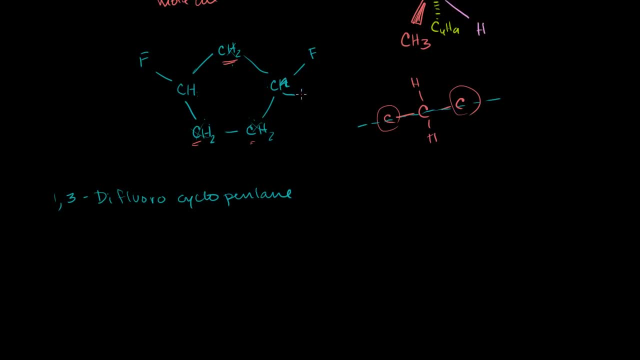 Because if we were to break it out a little bit, you could break it out like that and break it out like that Instead of writing a CH. actually show the bond to the hydrogen, And this guy is bonded to one hydrogen, one fluorine. 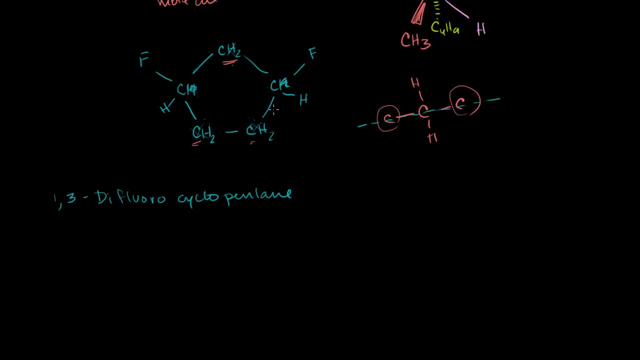 And then if we were to work our way around the cycle, and these cyclical, these cyclic molecules are a little bit. it's sometimes a little tricky to identify whether you're bonded to the same group or different groups. But actually, let me not make it too messy while we try to figure this out. 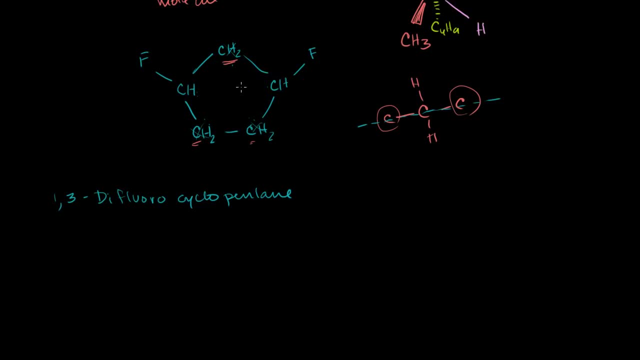 To figure out whether it's bonded to the same group. let's kind of take a walk around the cycle, around the cyclopentane ring. If we go this way, if we go in a counter, Let me do it in a different color. 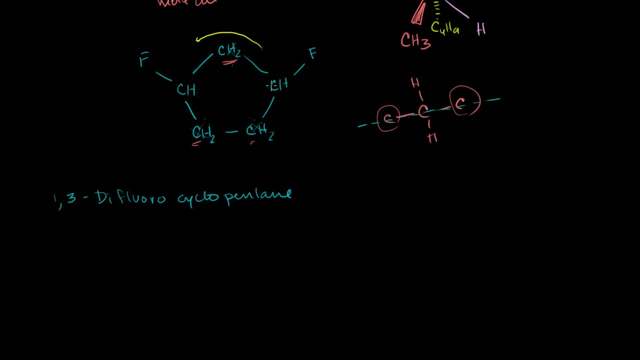 If we go in a counterclockwise direction from the carbon in question, we're going to hit a CH2.. Then we're going to hit a CH. So we're going to hit a CH2, then we're going to hit a CH. 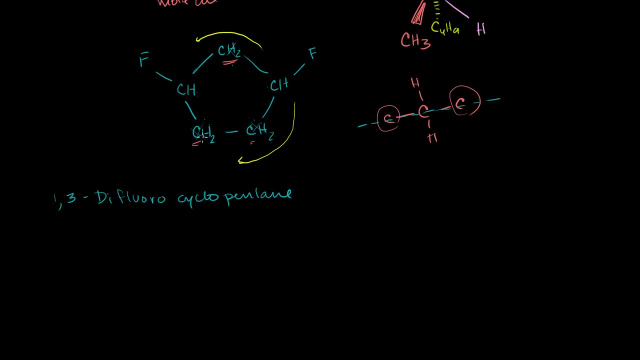 If we go this way, we're going to hit a CH2, and then we're going to hit another CH2.. So this guy is fundamentally- this bond is bonded to a different group than that bond up there is, And it's also bonded to a hydrogen, also bonded to a fluorine. 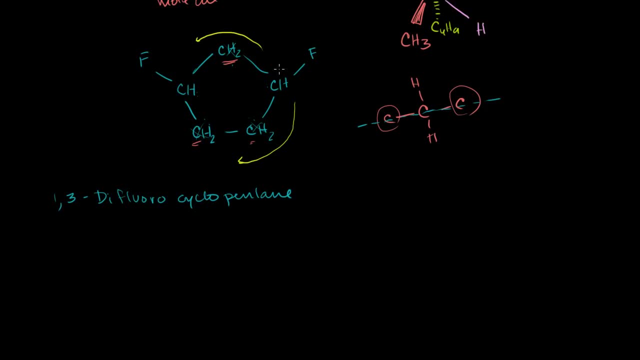 So this is bonded to four different groups. So this is a chiral carbon. So that is a chiral center. Chiral center. Now, the exact same argument can be made for this carbon right here. You can make that exact same argument that. look if you were to walk counterclockwise from this. 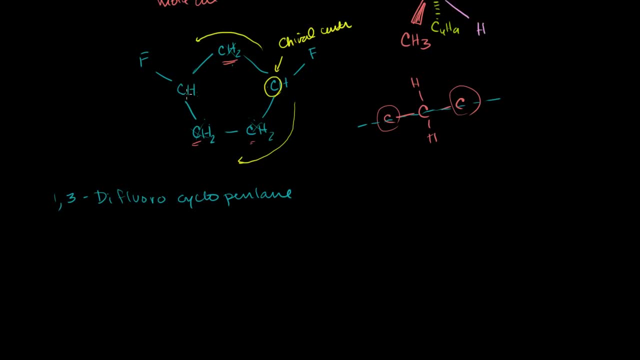 or if you were to walk counterclockwise, you'd hit a CH2, then a CH2.. If you were to go clockwise, you'd hit a CH2, then a CH, which happens to be connected to a fluorine. 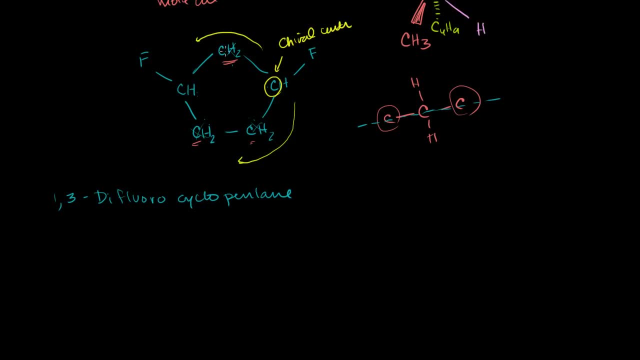 So you're actually going to see something different depending on whether you're going down that into that group or into that group. And then it's also bonded to a hydrogen And a fluorine- Four different groups. This is also a chiral center. 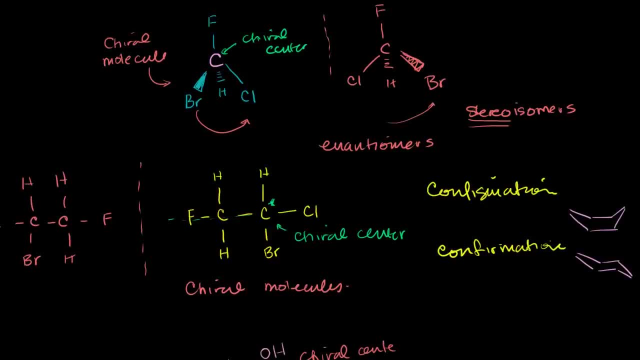 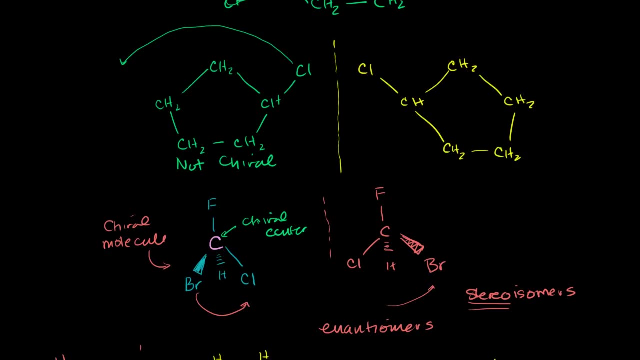 Another way to think about it and it's actually interesting to compare it to this molecule up here which was not chiral and did not have a chiral center, This molecule up here- and let me draw a little different to make it a little bit more clear- 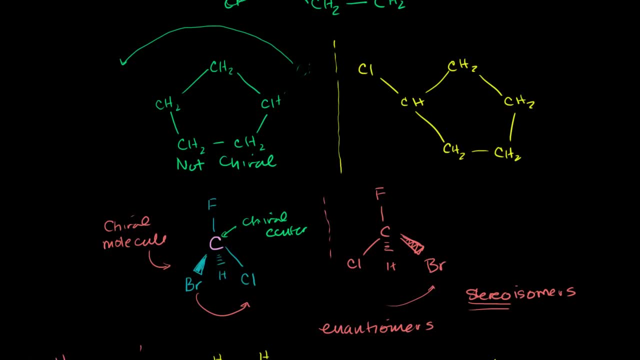 Let me draw it a little bit different. So this one I can draw it like this I'm just making: If you have the chlorine like that Over here, we thought about this as a potential chiral center and it's kind of playing the same role as in that example down here. 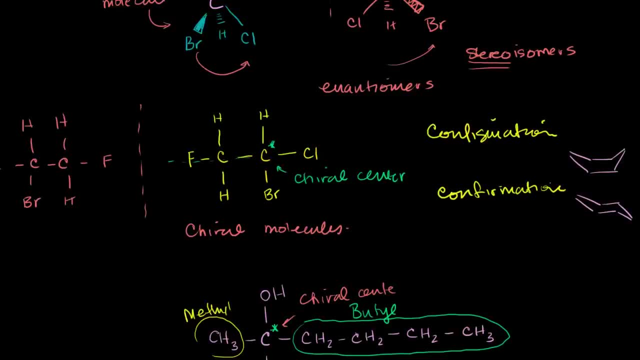 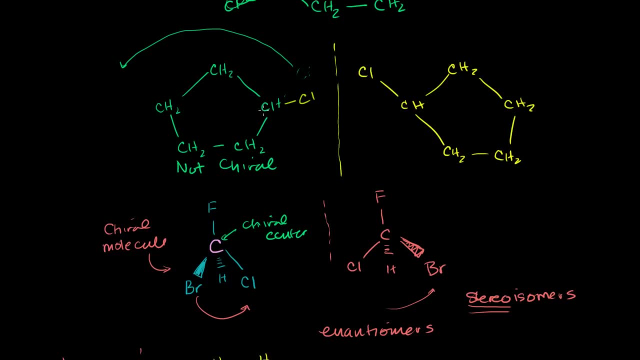 As in this example of this carbon down here. But you see, over here this is not a chiral center, because there's actually an axis of symmetry for this molecule that goes through that carbon. So you can actually just draw an axis of symmetry that goes exactly through that carbon. 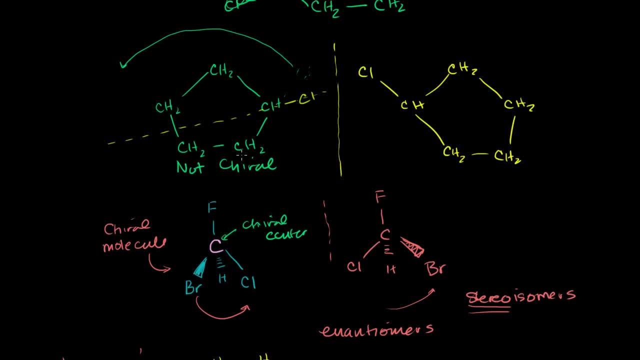 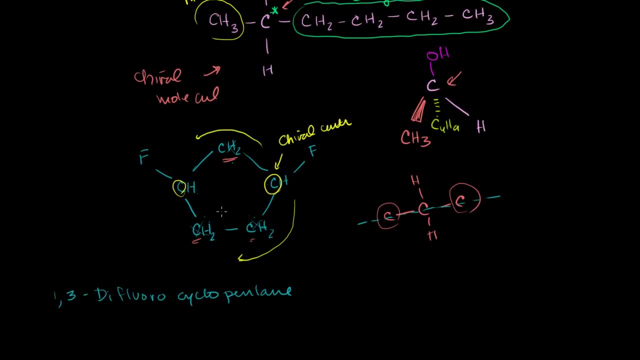 It's not. you know the way I drew it. it's not completely neat, But you can see that that is the reflection of that if I were to draw the bonds actually a little bit more symmetric Over here if we try to do the exact same thing. 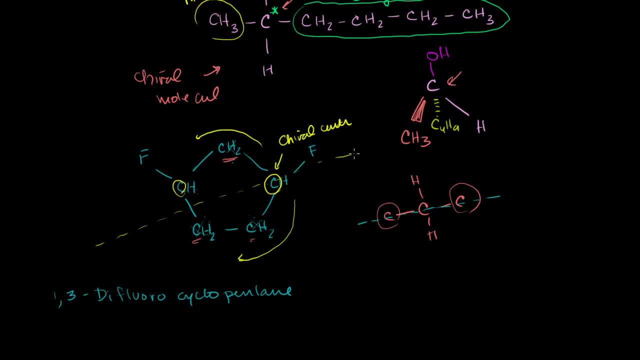 If we try to draw an axis of symmetry over here, If we try to draw an axis of symmetry, we can make that bond to the fluorine go through our axis of symmetry. We'll see that that still is not. this is still not the reflection of this, because we have a fluorine up here. 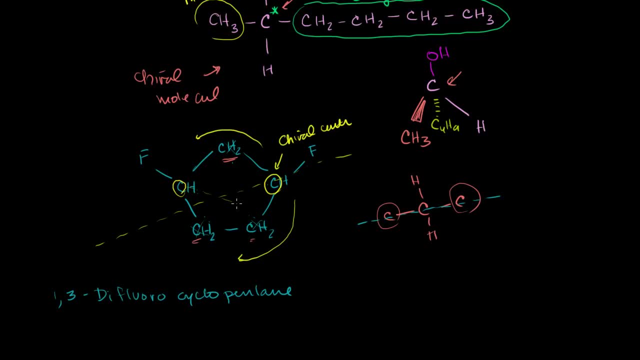 We don't have a fluorine over here, And we could do the same thing with this end. If you try to do an axis of symmetry, fluorine up there, no fluorine over here. So this is the reflection of that. So this, each of these, are definitely chiral centers, while this carbon up here, this carbon up here, was not a chiral center.